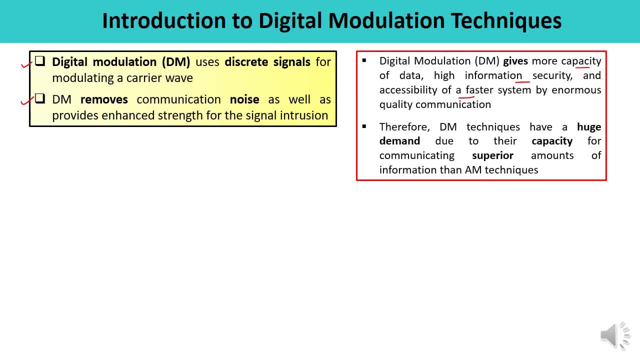 applications as well, and because of their capacity for communicating superior quality of information in comparison to the analog modulation techniques. So these are the various advantages because of which they are always preferred one. There are many types of digital modulation techniques and some of their combinations also exist, So, depending upon the 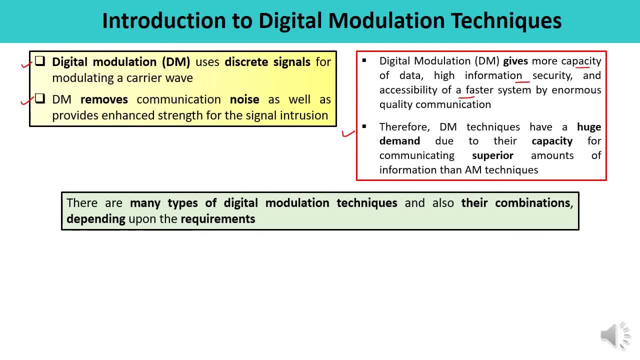 requirement of the combination. the modulation techniques can be utilized into a number of applications, But three basic techniques are there, Prominent. you can say ASK, that is amplitude shift king, FSK, that is frequency shift king, and PSK, or phase shift king. So in this video I will be talking about the phase shift king. 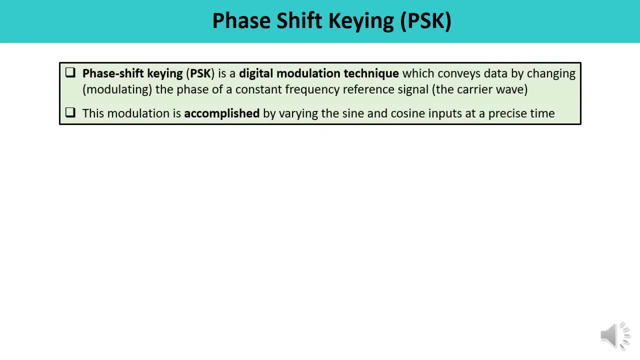 What do you mean by phase shift, king or PSK? How can you define it? PSK is a digital modulation technique and it conveys data by changing, that is, modulating, the phase of a constant frequency reference signal. This constant frequency reference signal is nothing but the carrier wave. 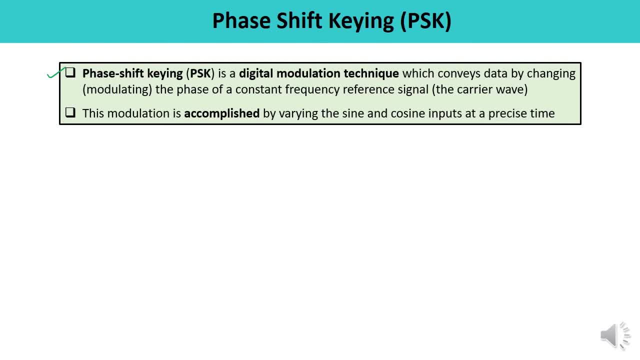 and this modulation is achieved by, or modulation is accomplished by varying the sine and cosine inputs at a particular time. So this is how this type of modulation is being achieved. Or you can define: PSK is a digital modulation technique in which phase of carrier signal is. 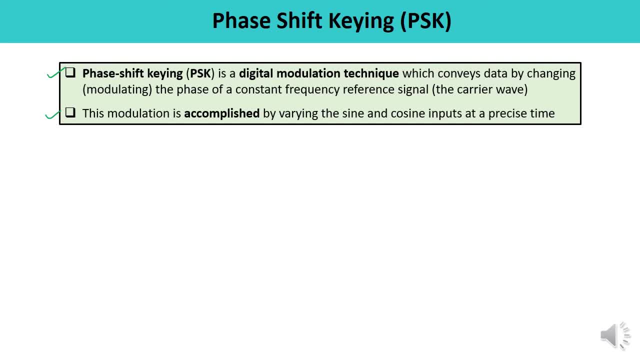 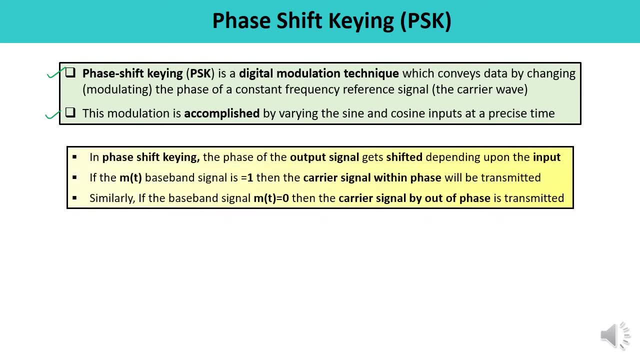 changed by varying sine and cosine inputs at a particular time. PSK technique that is widely used in a number of applications like wireless LAN, biometric contactless operations, along with RFID, Bluetooth communication, satellite communication, So there are various applications. 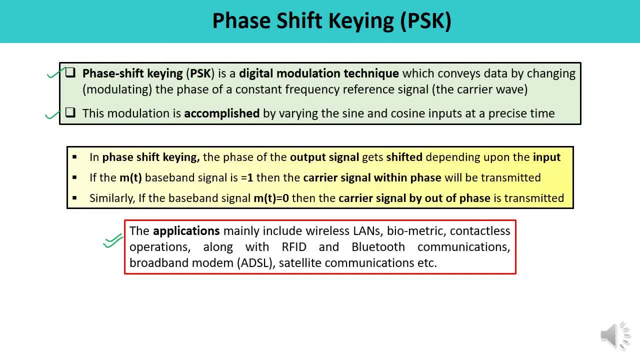 And in case of phase shift king, the phase of output signal gets shifted depending upon the input. So if empty it is equal to 1, means if the baseband signal is 1, then the carrier signal will be within phase and if it is 0, then the carrier signal will be out of phase which will be transmitted. 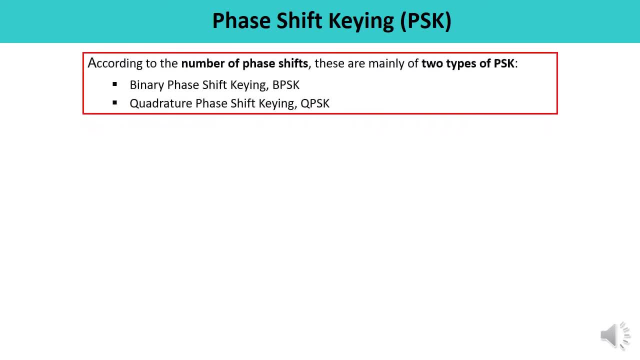 actually, According to the number of phase shift, there are mainly two types of PSK. First is binary phase shift king technique, that is BPSK, and second is the quadrature phase shift king, that is QPSK. So this is the classification which depends on the number of phase shift. So now let us talk. 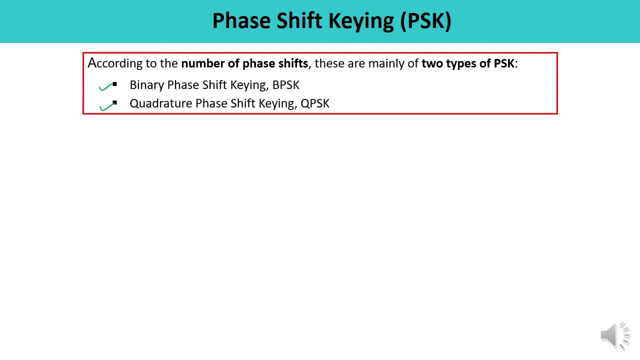 one by one in brief, and then I will be talking about the BPSK in this particular video. First, what is binary phase shift king? Binary phase shift king, this is also known as a two-phase PSK or phase reversal scheme. So in this technique, sine wave carries two phase reversals like. 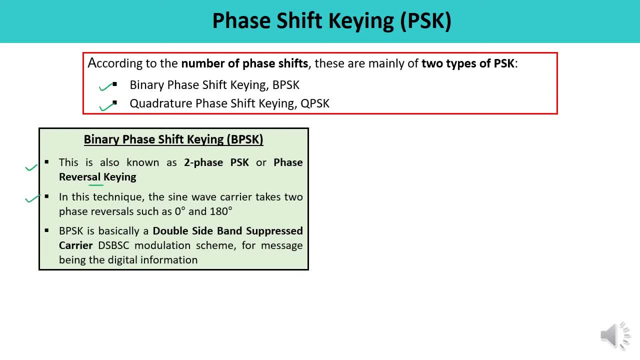 0 degree and 180 degree. that is why it is known as a binary two phase PSK and BPSK is basically a double sideband suppressed carrier DSBSC modulation, which you have already studied. So this is a double sideband suppressed carrier modulation scheme for a message being the 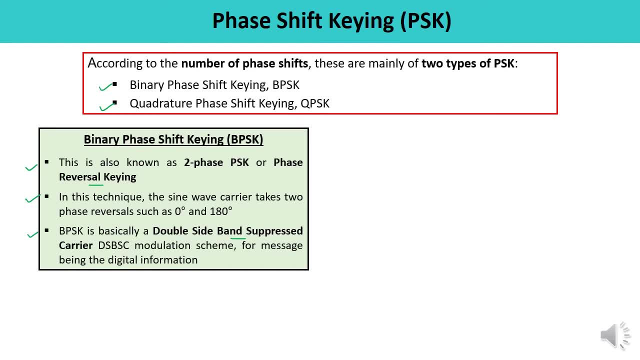 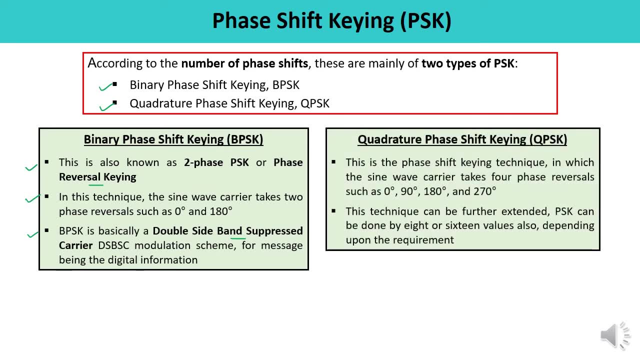 digital information. So here the information, which is the message signal, that is, in the digital form. Second is the quadrature phase shift keying. quad means four. So this is the phase shift keying technique in which the sine wave carries, sine wave carrier that takes four. 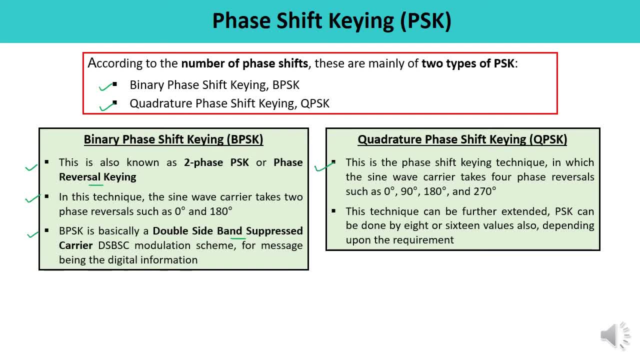 phase reversals. So this is the phase shift keying technique in which the sine wave carries and four phase reversals are 0 degree, 90 degree, 180 degree and 270 degree. So in this particular kind of technique, this particular technique which we are saying a quadrature phase shift keying, 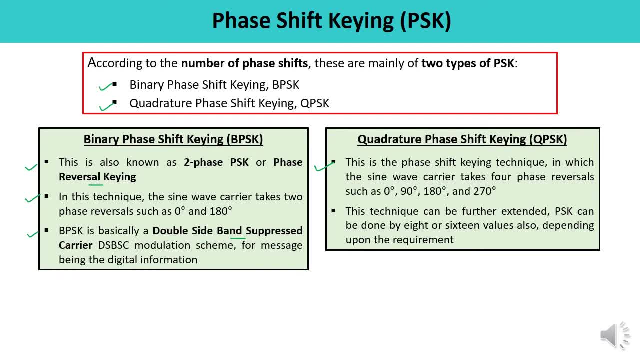 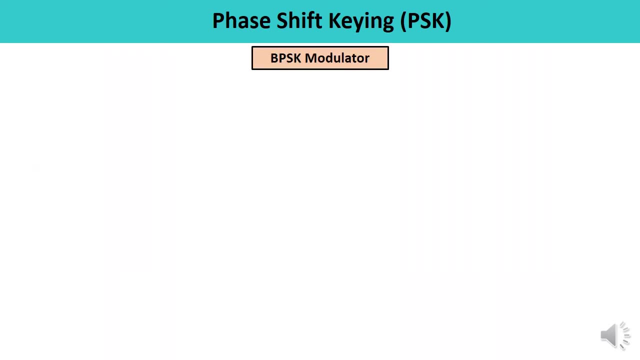 that can be extended further. So PSK can be done or can be accomplished by using 8, 16 values accordingly, depending upon the requirement. So this particular kind of technique, it can be extended further. So now let us talk about in detail for binary phase shift keying. So first you know what is. 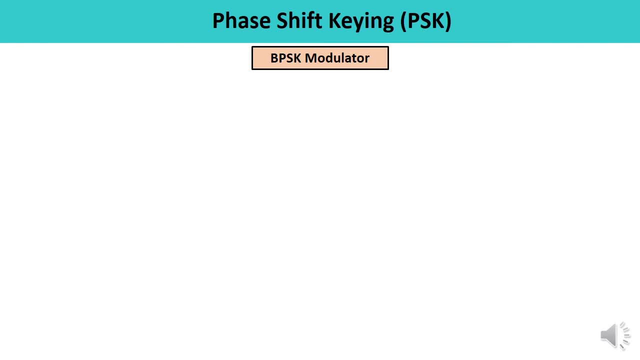 binary phase shift keying, or BPSK. that is also known as a two phase PSK or phase reversal keying. So now let us understand how the generation means modulation and demodulation- is being done. So first, this is the block diagram of a BPSK modulator. 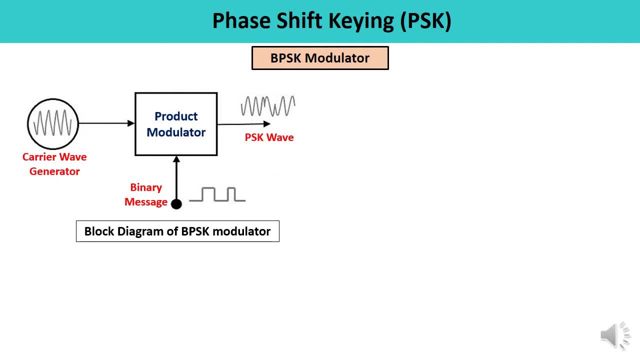 BPSK is binary phase shift keying technique. So in this diagram you can observe that it consists of a balance modulator, there is a carrier sine wave, carrier wave generator and the message signal like and message signal. that is the binary sequence. 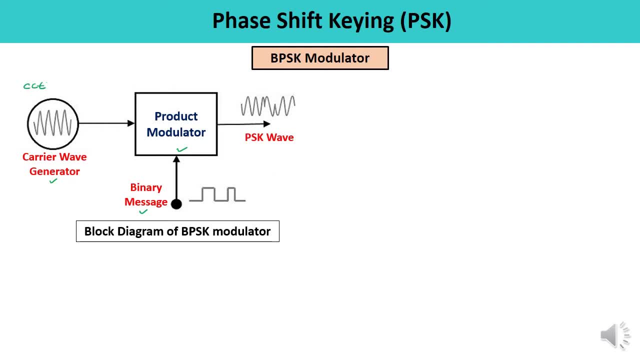 If we say carrier that is represented by CT, that is what if this is cos, omega, CT And the message signal is empty? So message signal will be what it may be: one zero, something certain combination, particularly So at the output you will be getting the BPSK signal means. 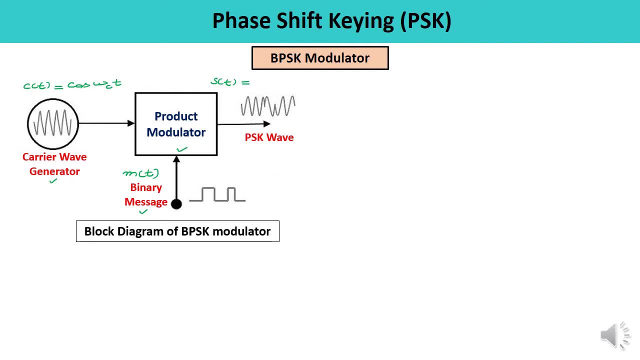 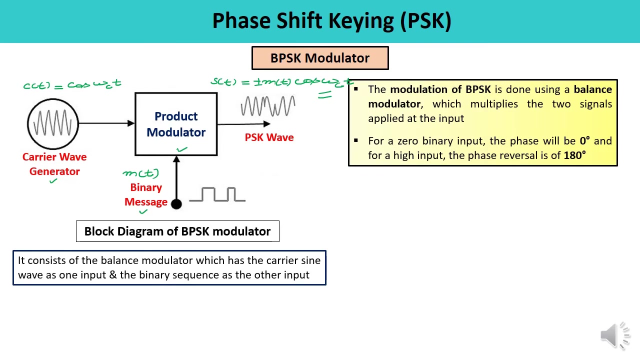 binary phase shift keying signal. So what you can write over here, ST is equal to what plus minus empty, depending upon the sine into cos, omega, CT. So this is what you are getting, the BPSK wave at the output. So here you must remember that the modulation of BPSK that is done by using 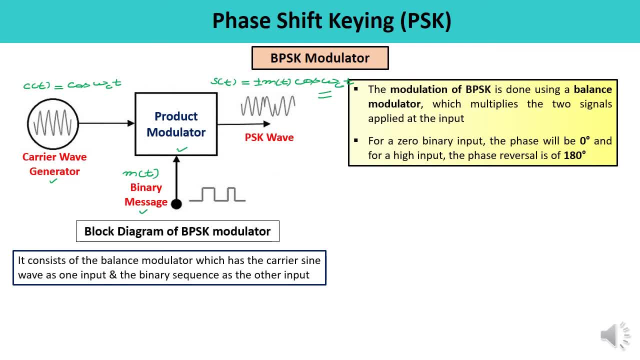 a balance modulator and the function of the balance modulator is to multiply the inputs which is being applied over here. And what is the input which is being applied? one is the carrier wave generator, carrier wave signal, and second is the message signal, the binary signal. So at the output you are 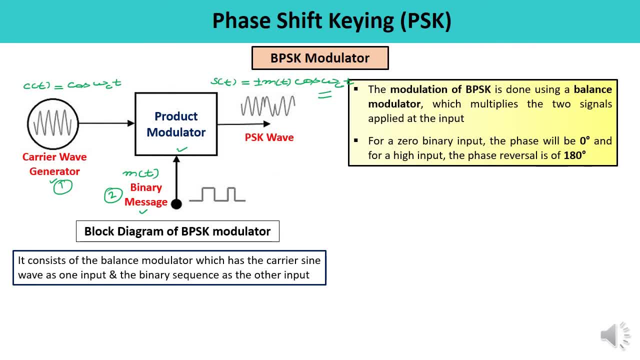 getting the product of these two binary input, the phase will be 0 degree and for high input, the phase reversal will be 180 degree, right? so this is how you can understand it, and you can now say how simple this is. this technique is very simple and accordingly you can draw the bpsk modulated waveform as well. you must be having 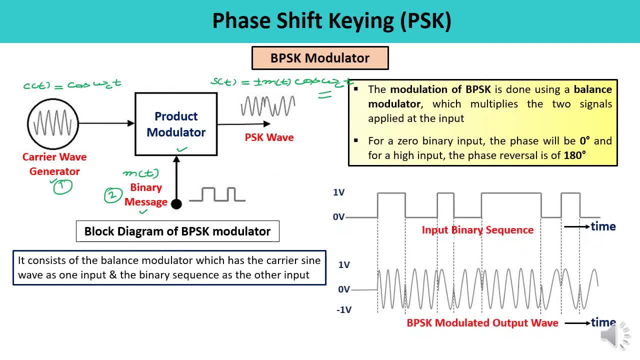 certain input binary sequence and accordingly you can plot the bpsk modulated output. so this is what the input binary sequence is being given over- here on the x-axis time is being taken- and input binary sequence that is a combination of 1, 0, something, and here you can observe in the binary: 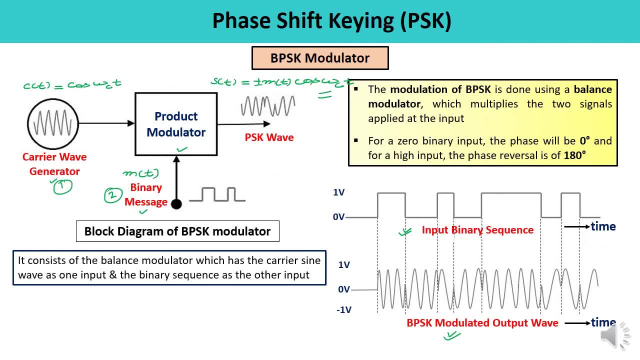 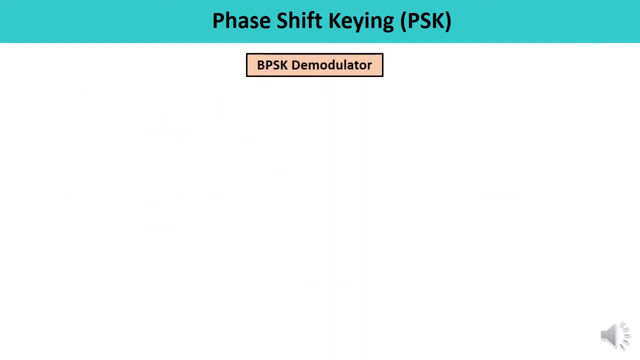 phase shifting modulated waveform, how the phase is being changed. so the output sine wave of the modulator, that will be direct input of the carrier, or the inverted means 180 degree phase shifted input carrier, which is a function of the dataset. So this is how you can explain the bpsk modulator. now let us talk about the bpsk demodulator, how the 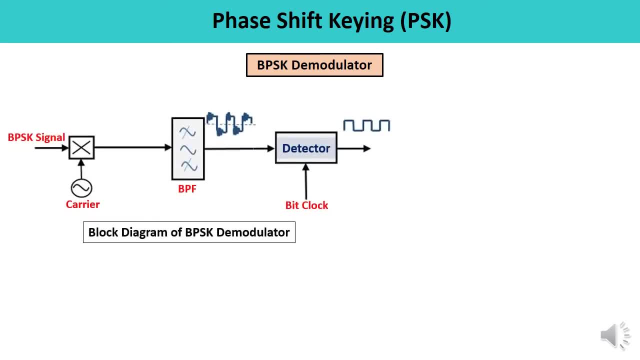 original signal is recovered back from the bpsk signal. so here you can observe the input of the input is the bpsk signal and from this signal the message signal is to be reconstructed or means required, one which is being received. so the overall, this demodulator, you can. 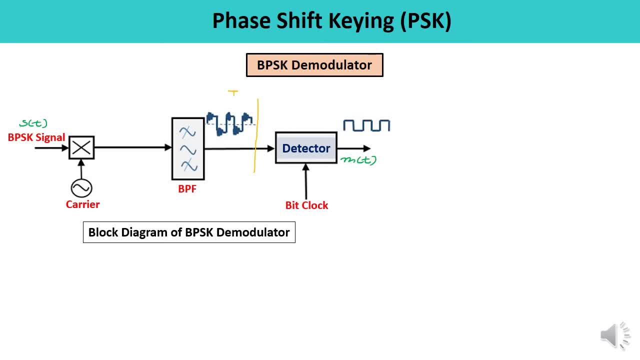 understand it by dividing it into two stage. this is the first stage and this is the second stage. so overall function you can understand like in this particular manner and if you observe this particular block diagram of bpsk demodulator, you can see there are there is a use of mixer local. 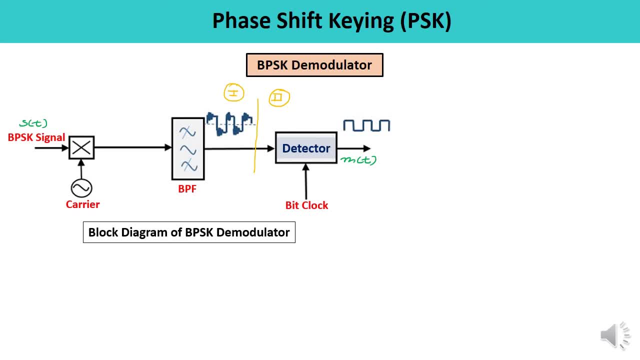 oscillator, bandpass filter and a detector. detector is the two input detector you can observe over here. the inputs to the detector are twoone is the output of the bandpass filter and second is the bit clock. and the output of detector is the original signal, which is the required one. so by recovering the bandlimited message signal here, 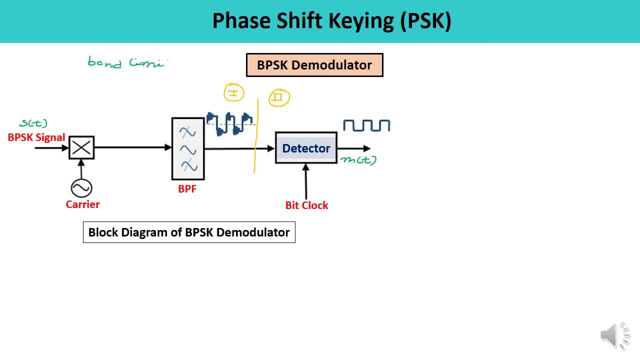 band limited signal is required to be recovered from the input stage and that is done by using this mixer circuit and the bandpass filter. so first stage of demod, first stage of demodulation, is completed at this particular point. So the baseband signal, which is band limited, that is, 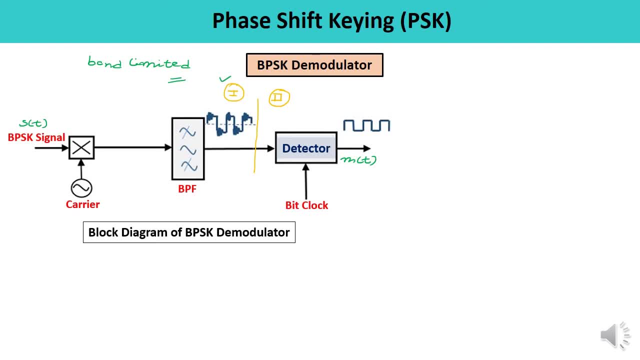 obtained and this signal is used to regenerate the binary message bit stream. means, with the help of this particular signal, binary message bit stream is to be regenerated. Now let us observe about the second stage. So in the next stage of demodulation, in the second stage, here, bit clock. 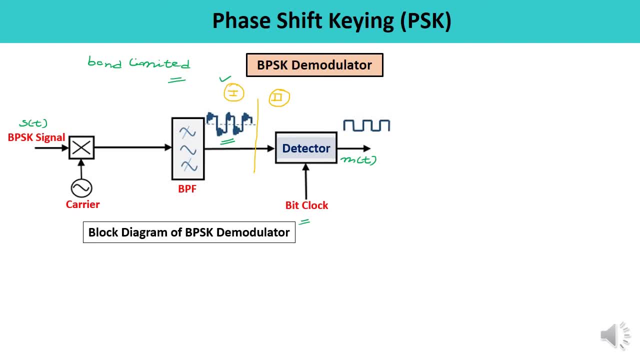 is already applied. So bit clock rate is required at the detector circuit to produce original binary message. signal means at the same rate If the bit, this particular bit, clock. if the bit rate is a sub multiple of the carrier frequency, then bit clock regeneration is simplified. So 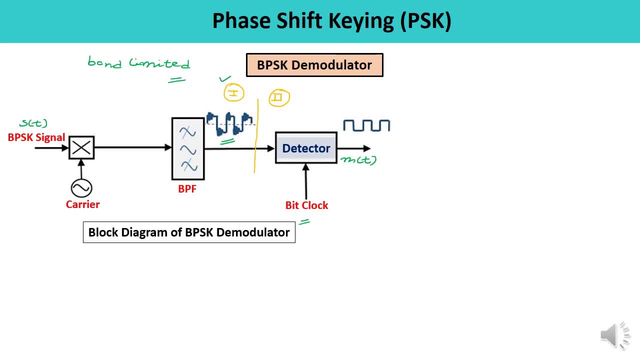 this is a required condition. this is a necessary condition that bit rate must be sub multiple of the carrier frequency right and to make the circuit overall to easily understand, there may be a use of decision making circuit it. that may also be inserted at the second stage of the. 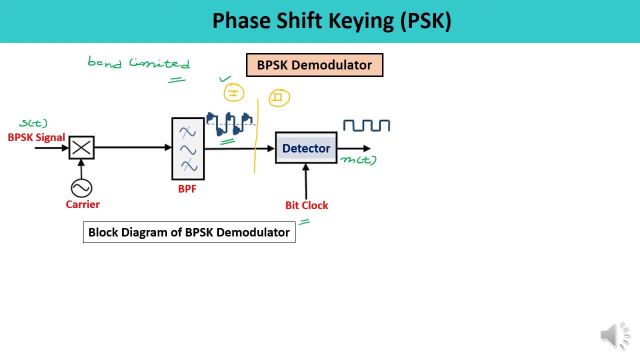 detection. So what is the function of the decision making circuit? So whatever the output is being like, achieved, that is to be compared with the threshold. if that is crossing the threshold level means that will be identified at the signal as a 1, otherwise that will be treated as a 0. So 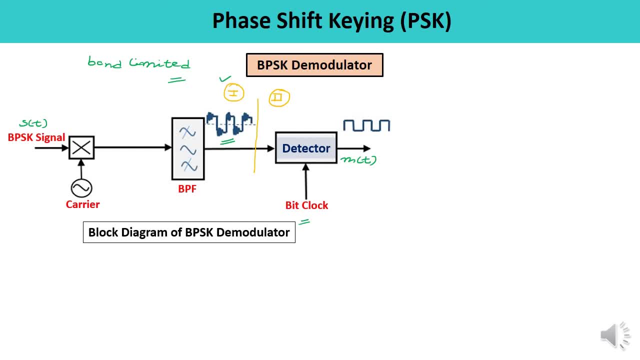 this is how you can explain this particular block diagram right Now. what is to be done over here if you have to derive the mathematical equation, how we are getting at the output and how to represent it. see, if we say we are getting YT, which is the product of this, and this ST is the BPSK signal. 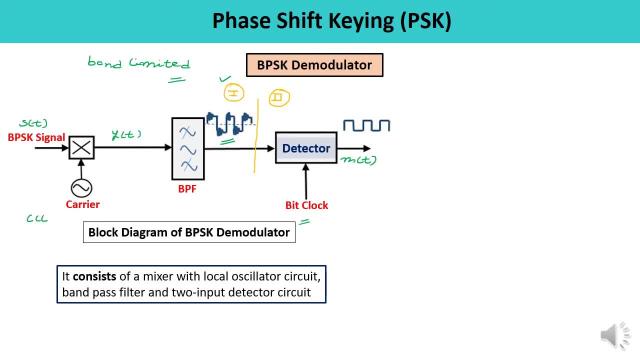 and the carrier signal, if carrier signal is represented by a CT. and what is CT? that is nothing but cos omega CT. So what you are getting at, the output YT, that is equal to what? ST into cos omega CT, ST already you know that is nothing. but this is M into T into. 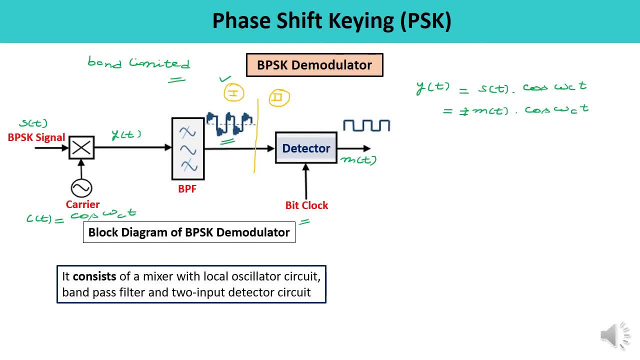 cos omega CT and into cos omega CT. So this particular term will be the square. if you simplify it further, you will be getting: this is nothing but empty, and this term will be what? 1 plus cos 2 omega ct upon 2.. If you expand this particular equation, what you are getting? 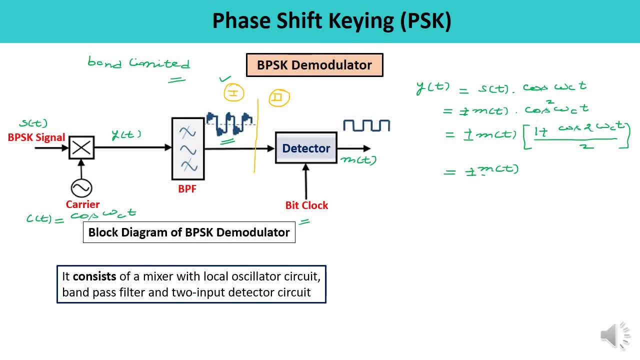 The first term will be plus minus empty upon 2, and the second term will be plus minus empty into cos 2, omega ct upon 2.. So here you can observe when it is being passed from the bypass filter and the detector, then at the output what you will be getting. The first component. 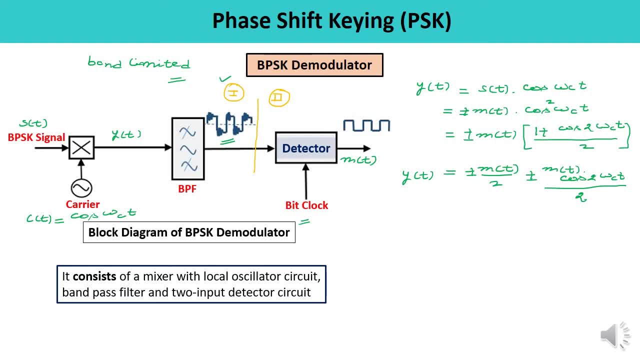 this particular plus minus empty upon 2, right this term at the output, you will be getting this term only, Which is nothing but the data. or you can say: this is the required information which is to be extracted over here. So this is how you can represent, how you can extract the original. 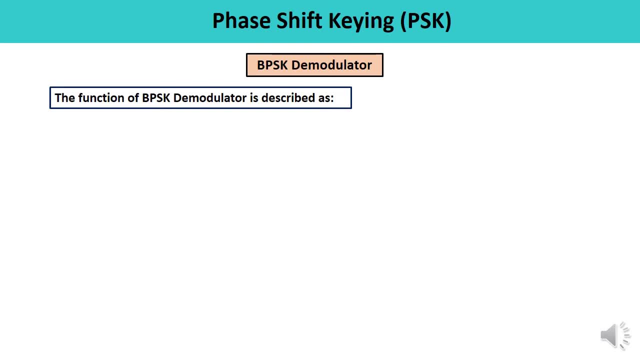 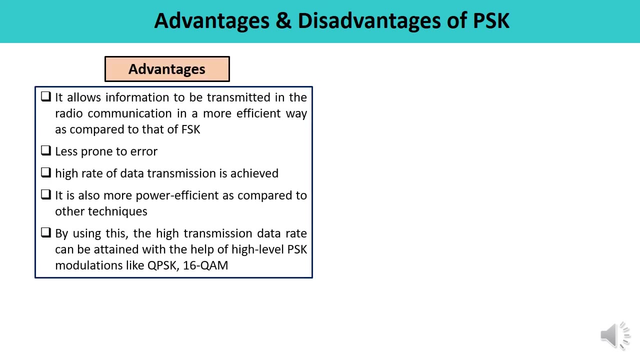 information. The function of BPSK demodulator is listed out over here. I have already explained. Now let us talk about the advantages and disadvantages of PSK. There are various advantages and some of them are: Phase shifting technique: it allows information to be transmitted in a radio communication in a more 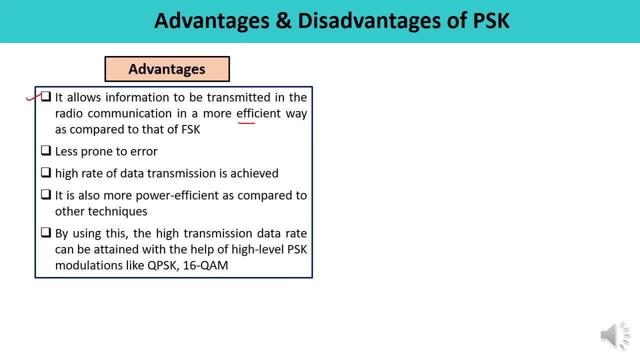 efficient way, The way of transmitting the information that is very, very efficient in comparison to the FSK. It is less prone to error, High rate of data transmission is achieved over here and it is also more power efficient in comparison to the other. So this is the way to. 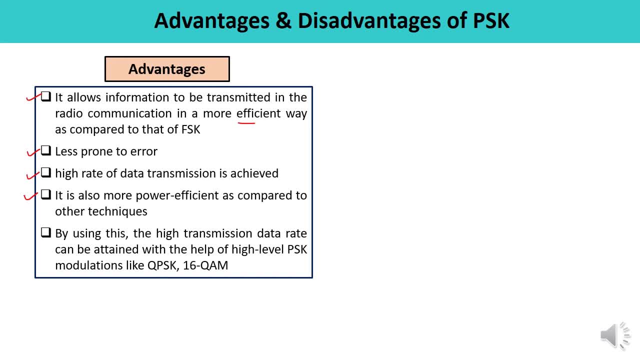 more other techniques if you compare it with the other model, a demodulation techniques, So it is also more power, efficient and by using this, high transmission data rates can be achieved with the help of high-level PSK modulation Like qPSK,16, qAM and so many other variants are also there. 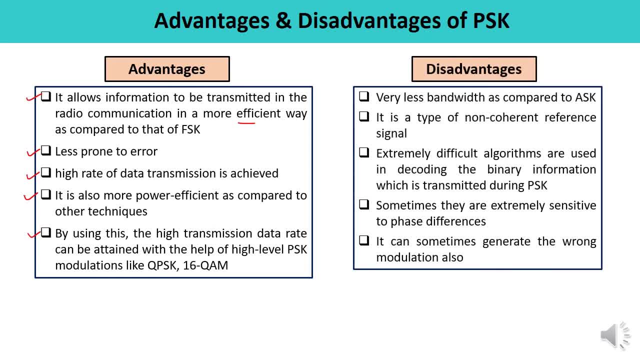 there are certain disadvantages also. It has very less bandwidth as compared to ASK Okay and it is a type of non-coherent reference signal. It is extremely difficult algorithm which is used to decode the binary information which is transmitted during the phase shifting technique.